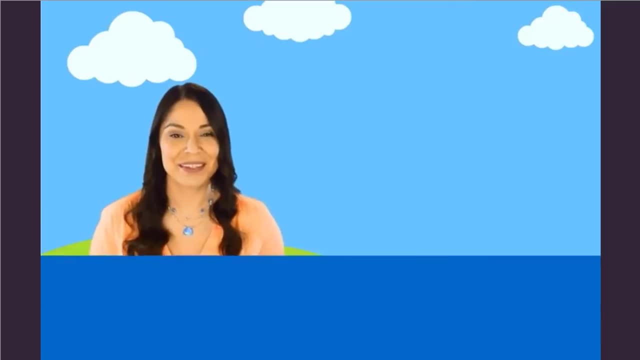 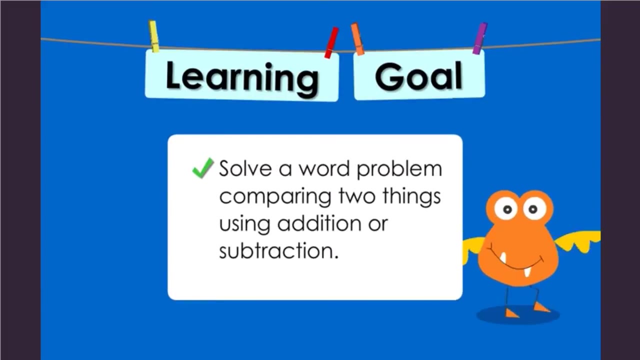 We're going to see who has more fish. Here's what we are going to learn about today. You will learn how to solve a word problem by comparing two things using addition or subtraction. Okay, we're ready, Let's go. Click the button to move on. 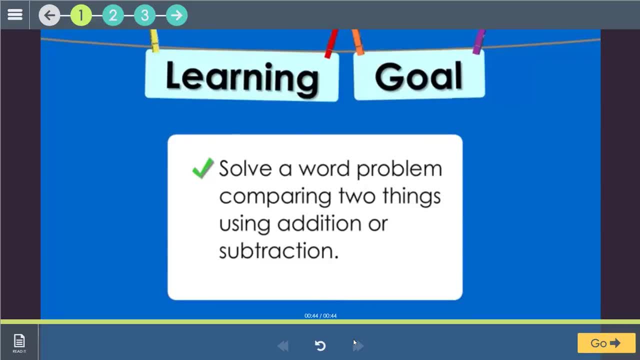 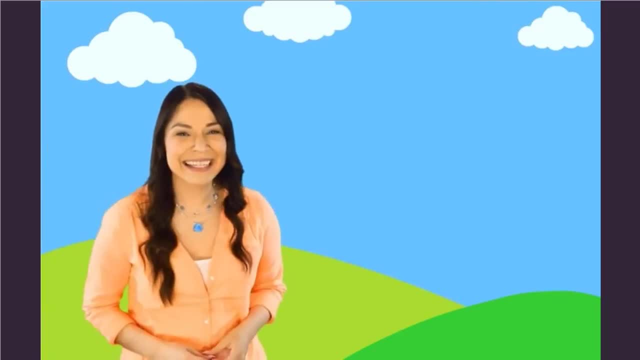 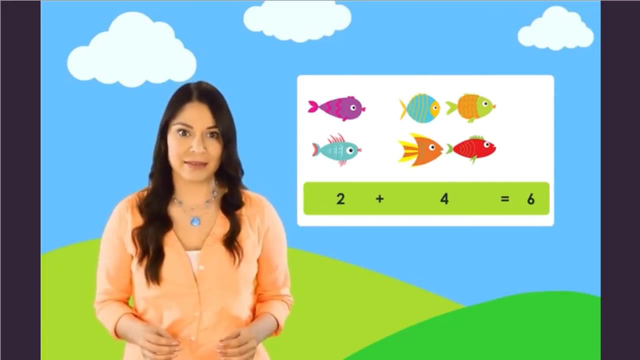 Time for Learning. lessons use a variety of styles to keep things fresh and diverse, and I really appreciate how many lessons include text, images, animation and real human instruction. Hi again, Let's talk about what you know. You know how to add by putting together two groups of objects. 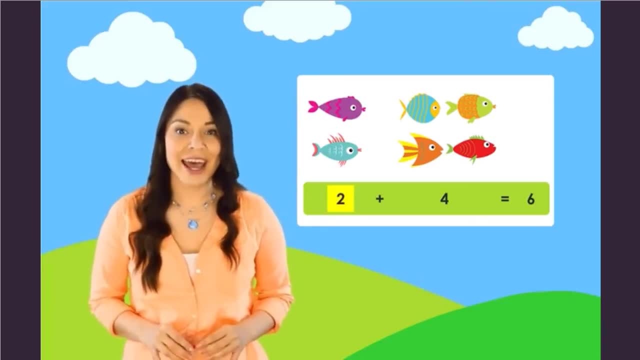 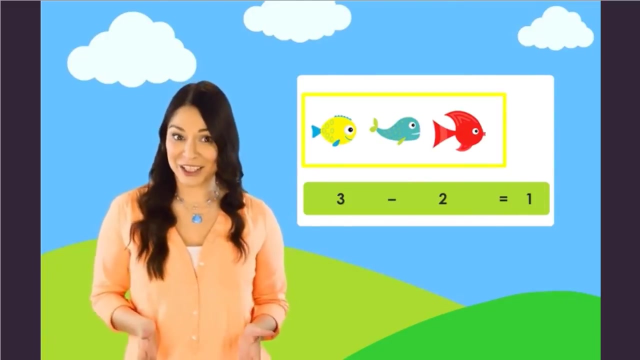 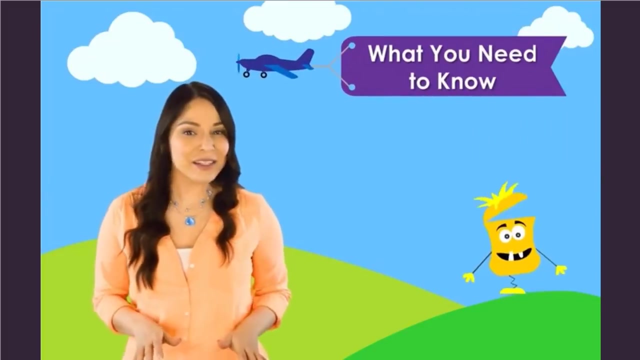 Like this: Start with two fish and add four fish. Two fish plus four fish are six fish, And you know how to subtract by taking away from a group. Here are three fish. Three fish minus two fish is one fish. Now let's talk about what you need to know. 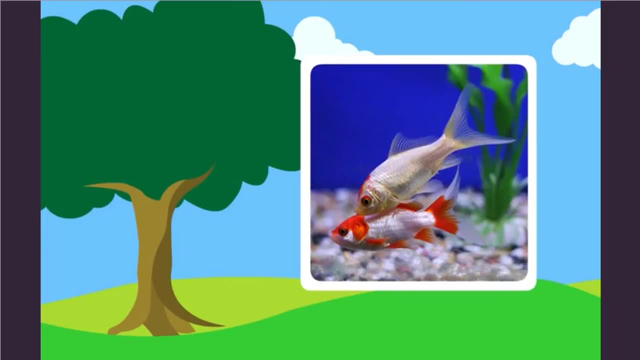 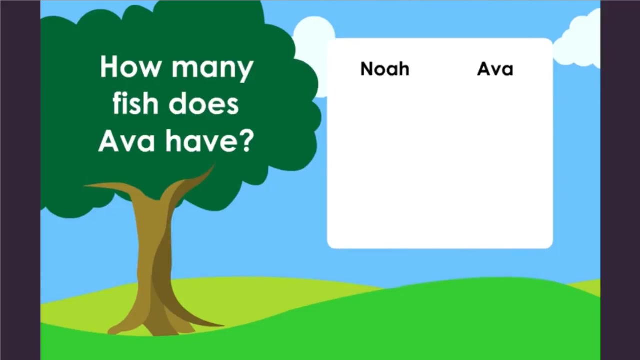 Noah and Ava each have pet fish. Noah has four fewer fish than Ava. Noah has two fish. How many fish does Ava have? Let's think about this problem. We know that Noah has two fish. This is for fewer fish than Ava has. 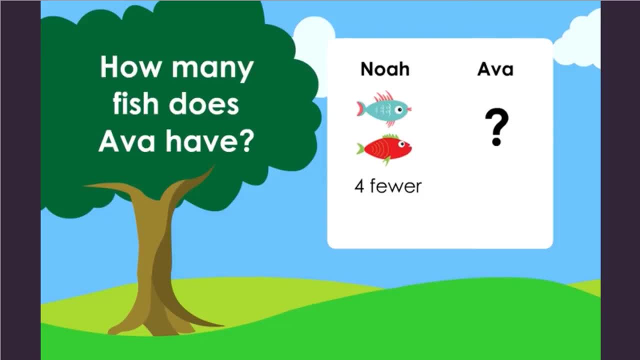 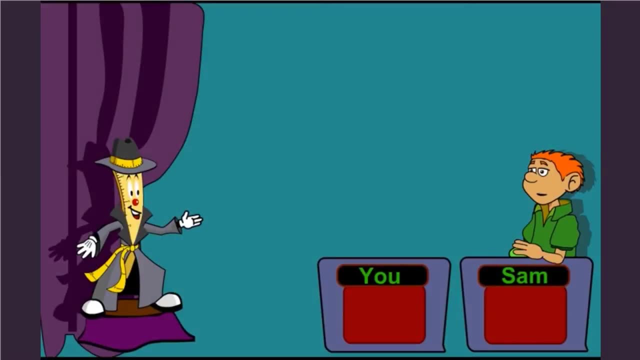 So who has more fish, Noah or Ava? Now we're making our way to the final lesson, where second graders will learn to tell time to the hour and half hour on analog and digital clocks. Welcome to another game of Power to the Hour. 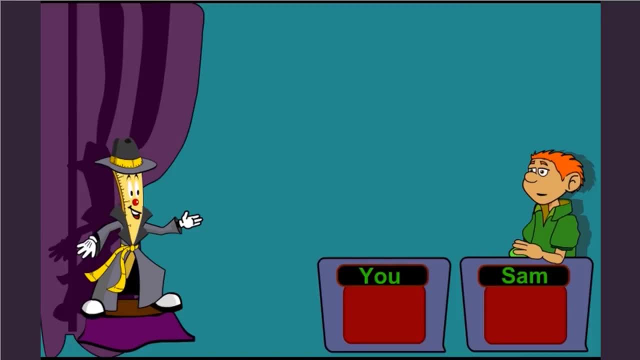 Today we have a new contestant going up against our audience. Welcome, Sam. Like most of the lessons, this one begins with a short introduction to the topic. Hi there, I'm a little nervous today. Mish, Relax, We will have a great time telling time. 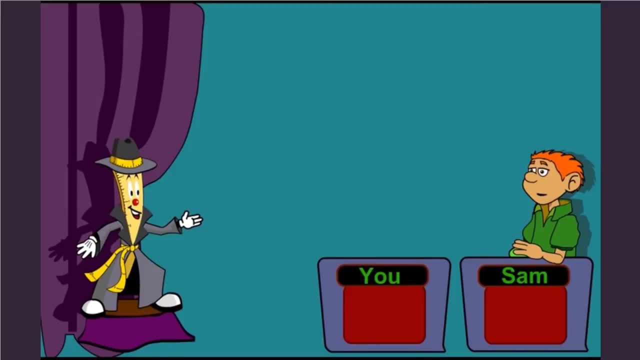 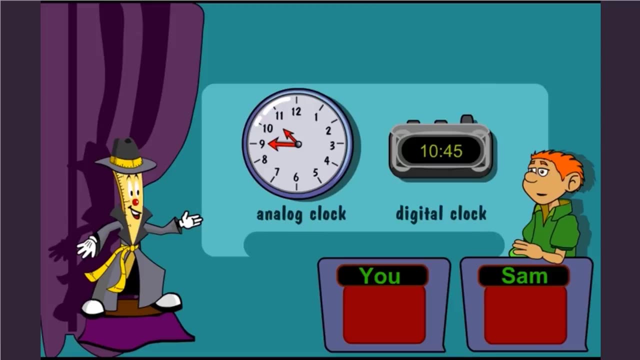 That's my problem: I'm not sure how to tell time. Not a problem, Our first round will help you. First let's review the parts of a clock. The clock has a minute hand and an hour hand. It shows the hours listed from 1 to 12..